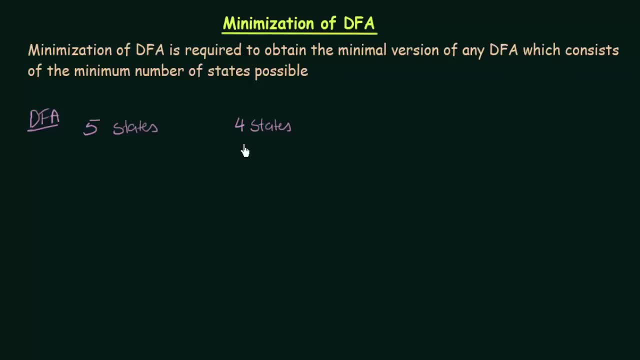 Both the DFA's are correct. Both the DFA's perform the exact same task, But one of them is designed using 5 states. Another is designed using 4 states. Both of them are correct, But here we see that the same DFA can be designed using a lesser number of states. 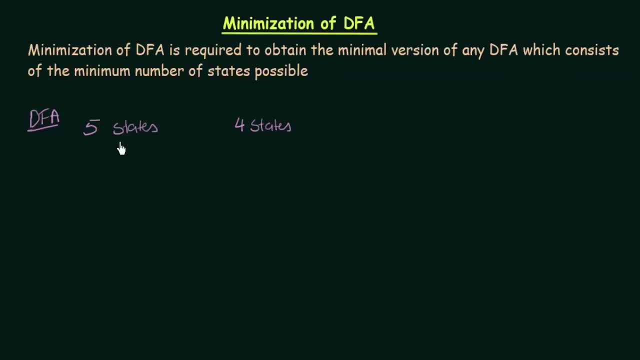 Now which one do you think is more efficient: 5 states DFA or the 4 states DFA? Obviously, it will be the one with the lesser number of states, So we want to design the DFA using the minimum number of states possible. 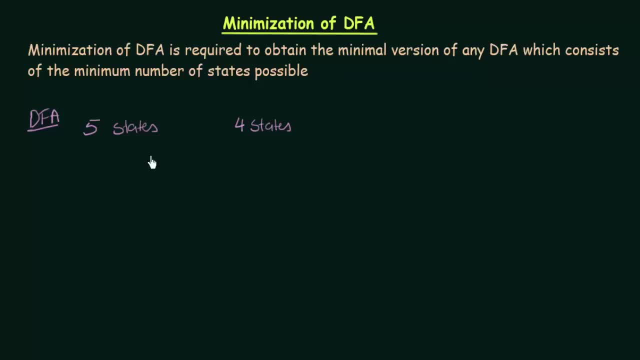 That is known as the minimal version of any DFA. Now, if you try to design a DFA directly in such a way to get the minimal version, it may be difficult for you. It is not impossible, but it may be difficult. It is possible only after you practice and practice. 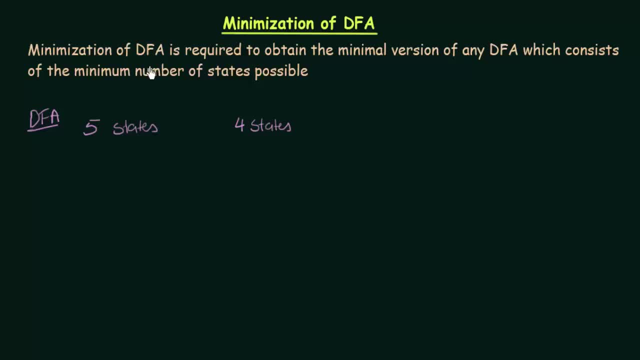 But there is a way of minimizing a given DFA. Given a DFA, you can apply some technique and minimize it and make it to the minimal version, And that is what we are going to study in this lecture. So how can we minimize DFA's? 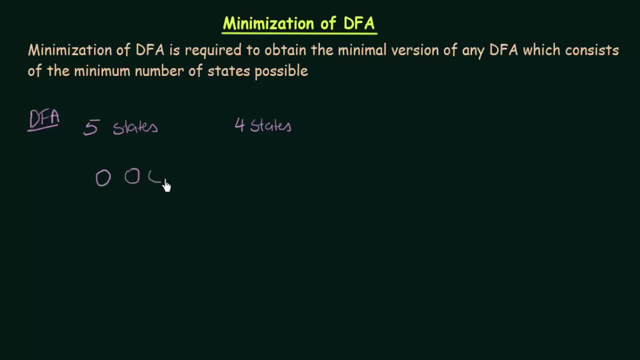 So let's say that you use these 5 states: 1,, 2,, 3,, 4, 5. You have these 5 states and you want to minimize this DFA. That means you want to reduce the number of states. 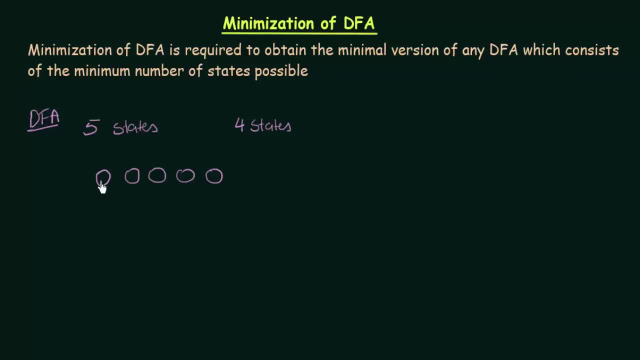 But keep the DFA performing the same thing. So how can you do this? What you can do is you can combine 2 states. Let's say these 2 states, you combine them together and you make this a single state. 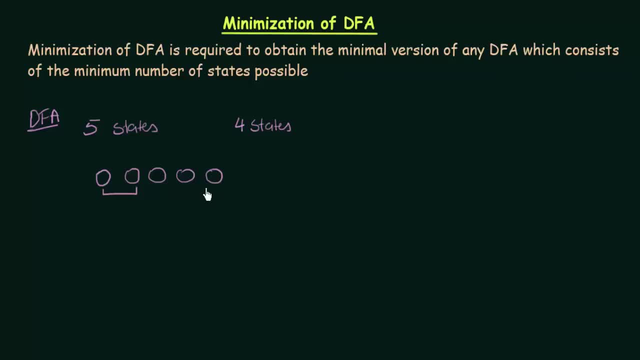 And then now you have 1,, 2,, 3,, 4 states. So that is how you can minimize it. But how can you simply combine 2 states? You cannot just simply combine 2 states. There is a condition when you can combine 2 states. 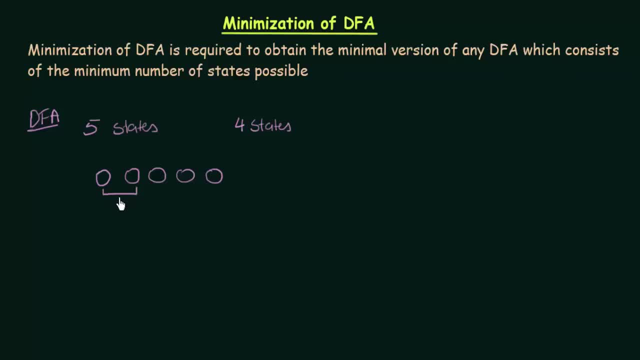 And what is that condition? 2 states can be combined. 2 states can be combined only when these 2 states are equivalent, When they are equivalent. Now, when are 2 states said to be equivalent? What is the meaning of equivalence? 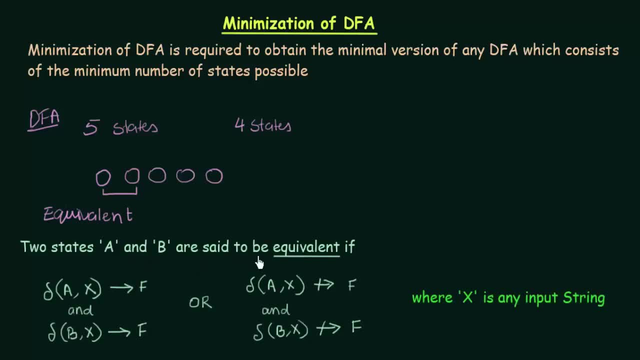 2. states A and B are said to be equivalent if A on getting a particular input string X. Here X is any input string. So if the state A on C is equal to DFA, getting the input string X goes to a final state. 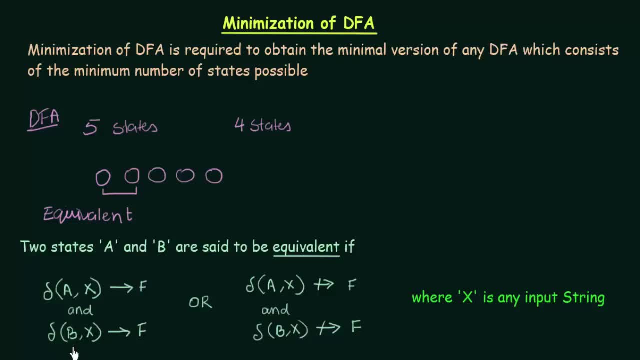 And at the same time if state B also, on getting that same input string, goes to any of the final states, then A and B are said to be equivalent. Or if A on getting an input string X does not go to the final state, 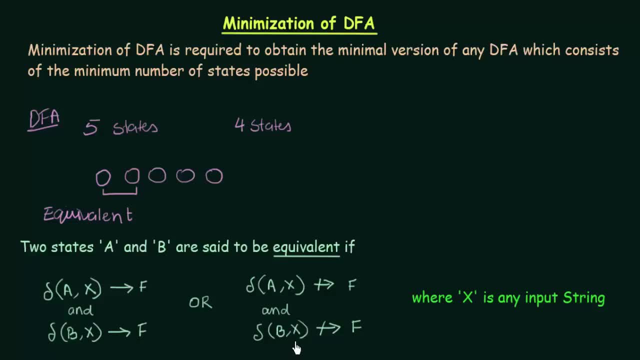 Then also B, on getting the particular input string X does not go to any of the final states. Then also A and B are said to be equivalent, And this will become more clear to you when we take some examples. And now what we have to study is types of equivalence. 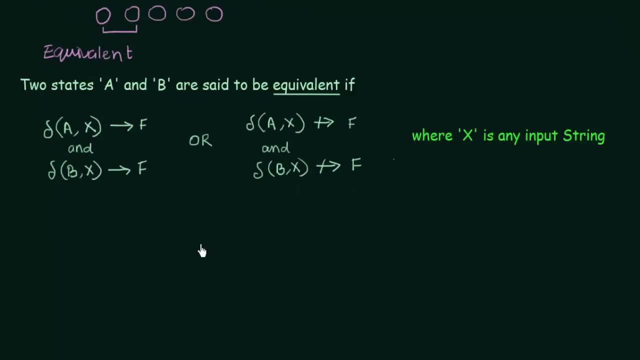 There are some different kinds of equivalences, like 0 equivalence, 1 equivalence, 2 equivalence, and so on. So next we will be seeing equivalence. What is that? So here we see that if modulo X equal to 0, this means that if the length of the string 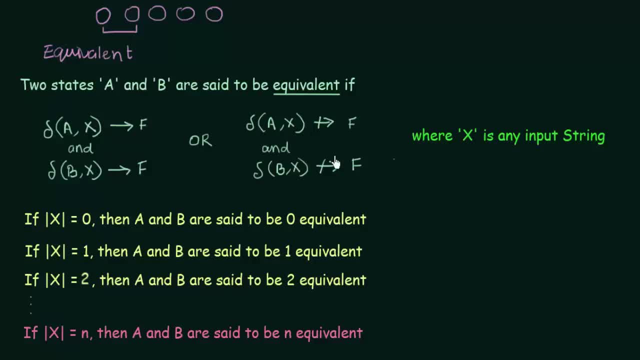 X. here we have taken X as any input string. If the length of that string X is 0, then A and B are said to be 0 equivalent, alright. And if the length of X is equal to 1, then A and B are said to be 1 equivalent. 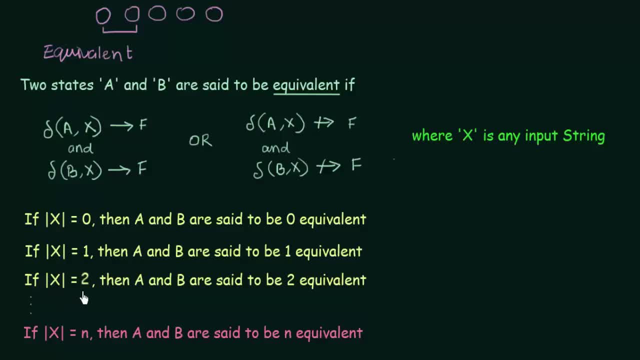 And if the length of string X is equal to 2, then A and B are said to be 2 equivalent. So in general we can write that if the length of the string X is equal to n, then A and B are said to be n equivalent. alright. 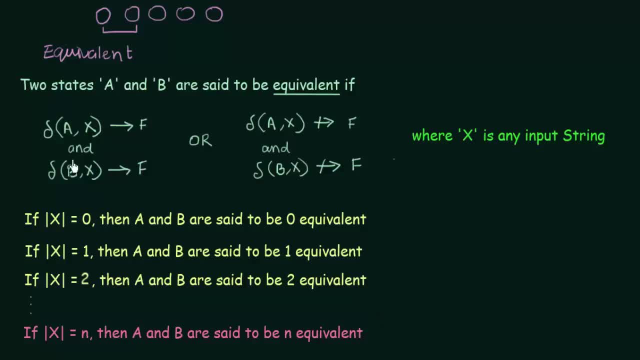 So these are the type of equivalences that we have And we already studied. when are two states, A and B, said to be equivalent? it is with these conditions: When, on seeing a particular input string, X if both A and B either goes to the final.